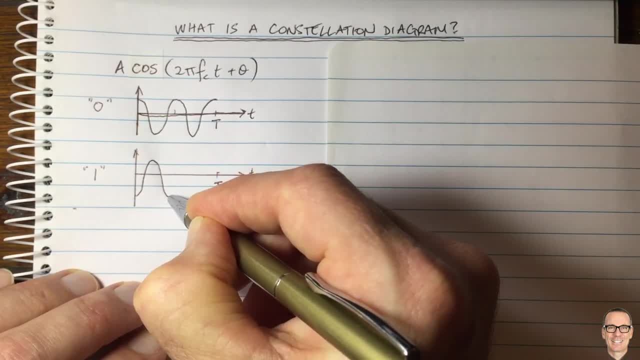 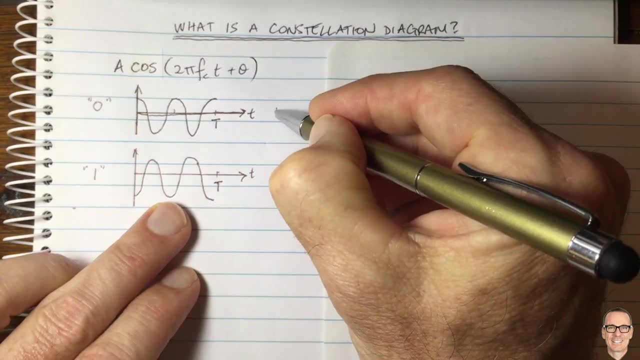 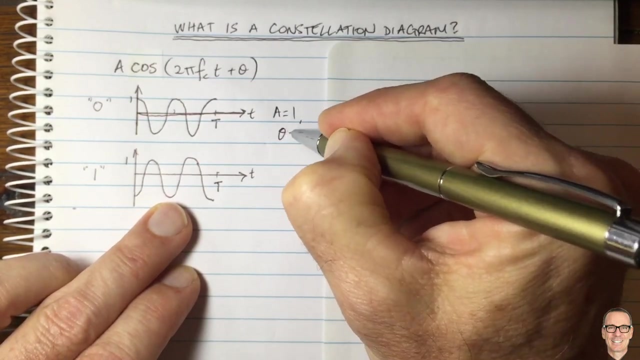 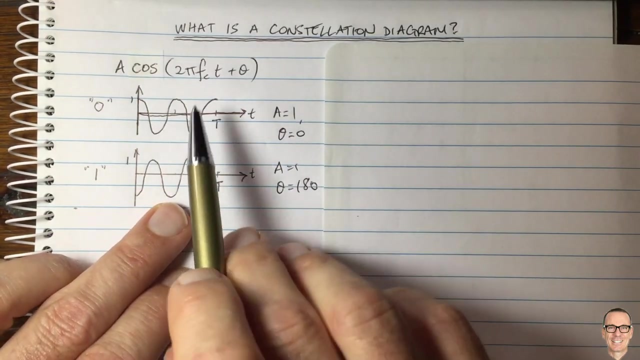 phase to represent a digital one. So we could represent this waveform to represent a digital one. So this waveform has a equals one, So we're going to have the same amplitude for both of them in this case and the phase equals zero, And this one has amplitude equals one and the phase equals 180.. And so you can see here, this is the waveform that actually gets sent from the antenna and oscillates the antenna at a 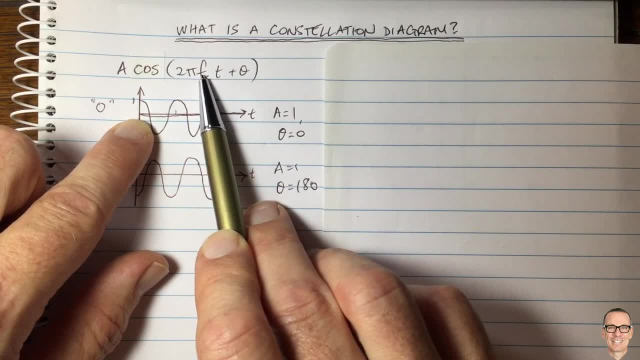 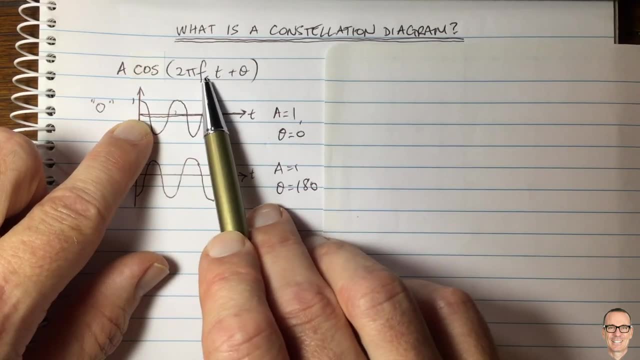 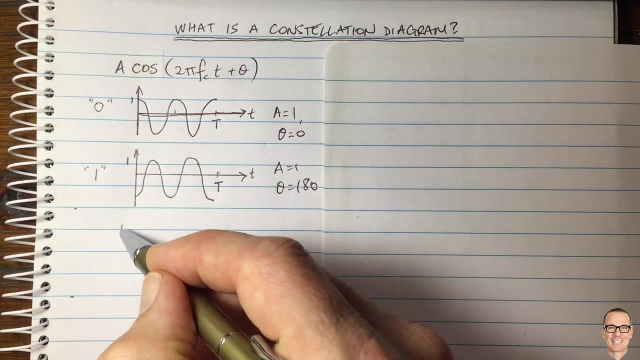 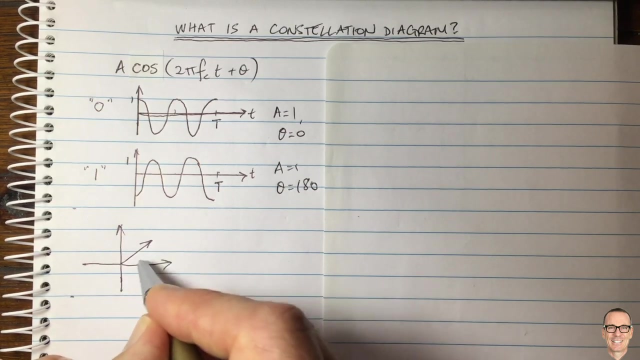 frequency that that antenna can radiate. So the FC has to be matched to the bandwidth that you're allocated in spectrum, and then you need an appropriate antenna. So this is a fixed value. So what you've got to choose is the amplitude and the phase. So that's two variables, And we immediately think about this on a amplitude and phase plot. So, for example, here's a vector. this vector has an amplitude of A and a phase of theta, And this is 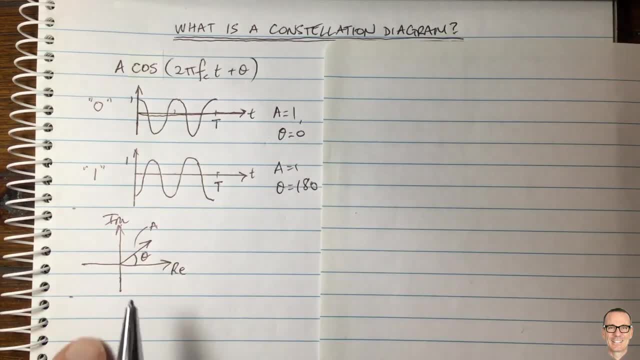 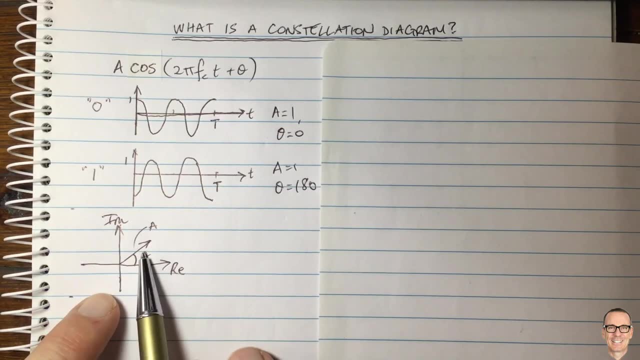 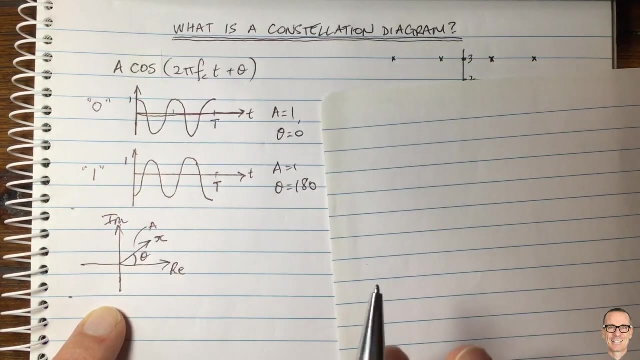 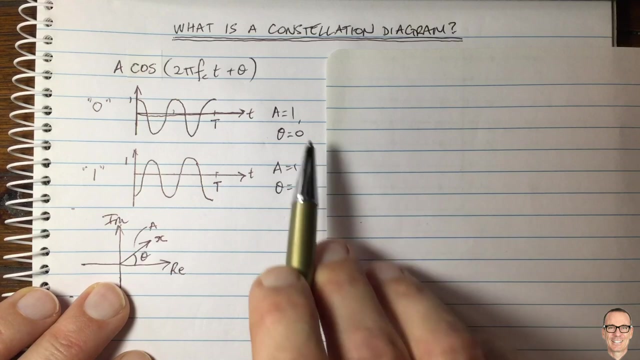 also can be represented in Cartesian with real and imaginary. Okay. so what are these two points in this amplitude and phase, or real and imaginary space? Well, we think of them as a vector and we're going to call that vector x. So that's how transmitted signal is going to be represented by this vector x And we can think about the different values this can take, And we've already got two of them here. if you're sending binary information- And this is already- 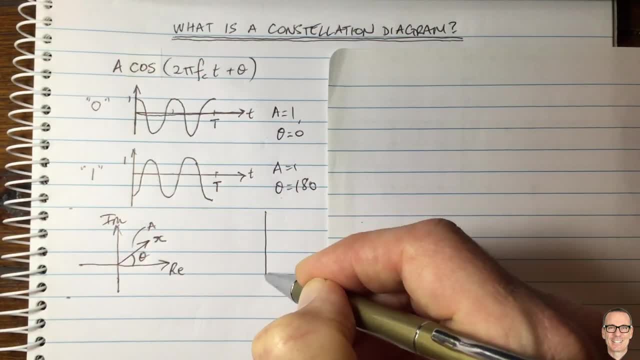 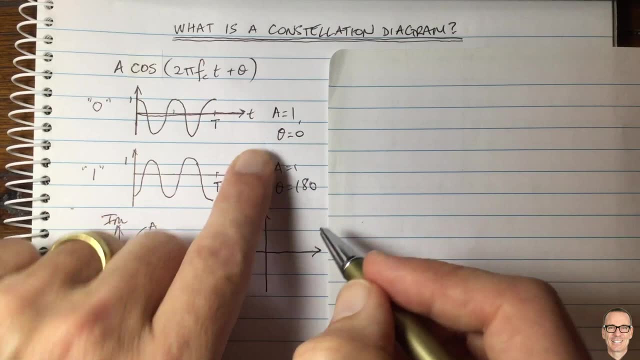 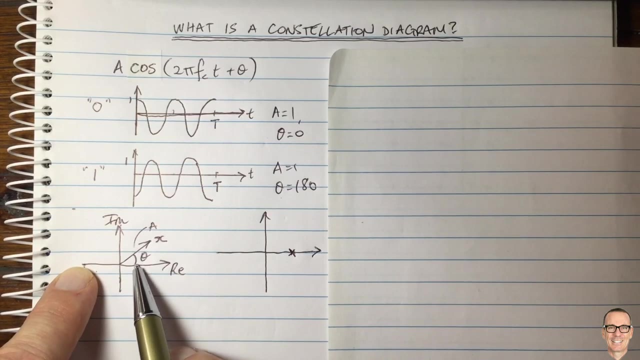 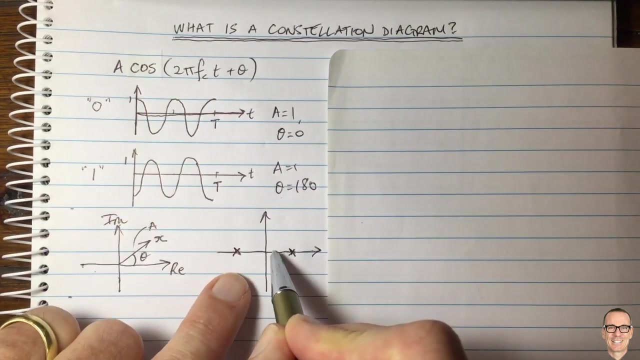 giving us what we call a constellation diagram. So in this simple case that I've shown here, where there's binary, then we've got these two possible values for x. One is here, so the amplitude equals one and the phase equals zero, because we count the phase from going in an anticlockwise direction, starting at the real axis. So that's this point here. And then the other point also has an amplitude of one, but a phase of 180 degrees, And this is our other possible value of a. 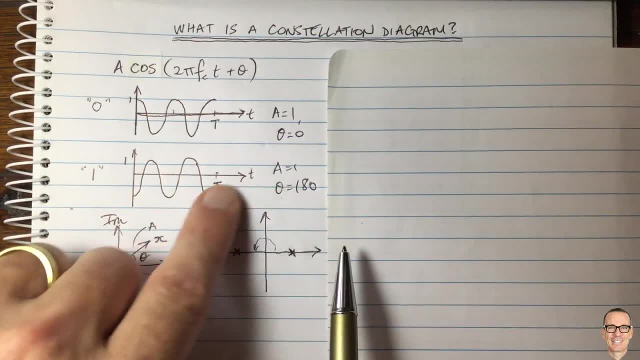 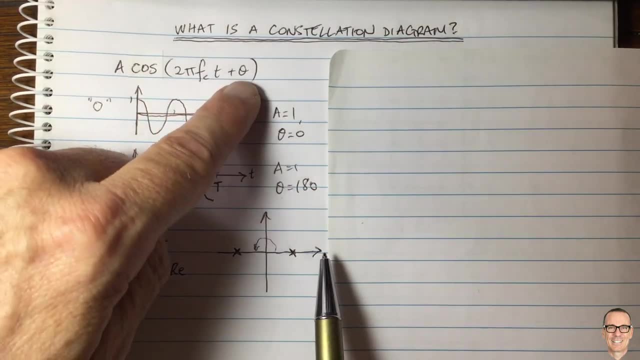 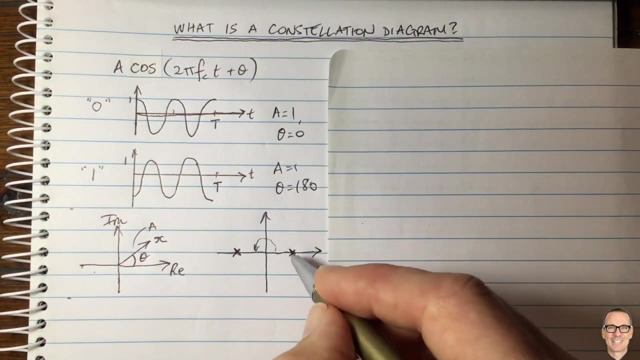 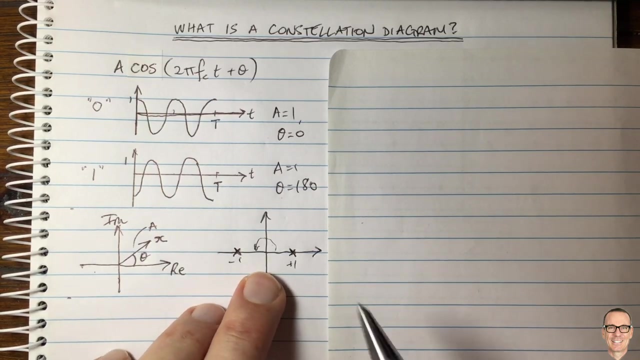 of x, that represents the waveform that we're sending. So this is what we call the constellation diagram for binary phase shift keying, because we're using the phase to encode the data. Both of these have the same amplitude, but we're using the phase to encode the data. So this is plus one and this is minus one. Okay, so what about something a bit more complicated? Well, if you wanted to have more than one bit per symbol. so this is called a symbol. we use that word for symbol. 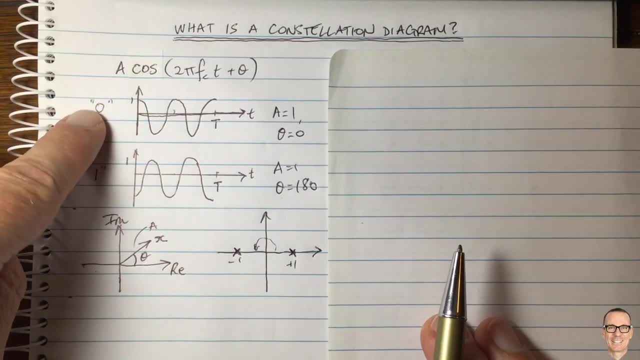 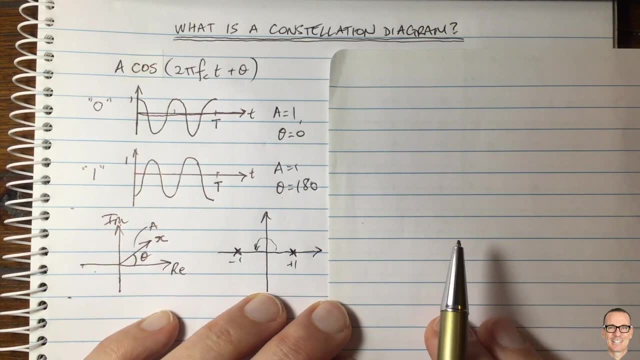 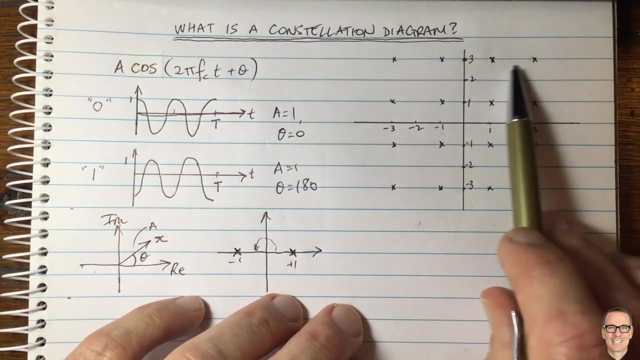 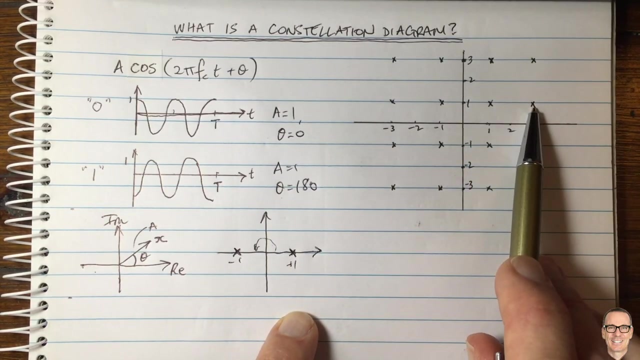 to transmit the data. you could group the data into multiple bits, into groups, and then instead of just needing two waveforms, you would need more waveforms. So let's say we group them into groups of four bits, then we would need 16, two to the power of four different constellation points. So this is our constellation diagram And these are what we call constellation points, And each one of these x's in this diagram here, where there are 16 points, because we're representing four. 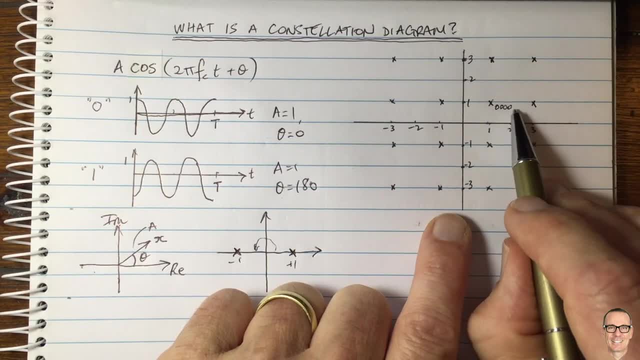 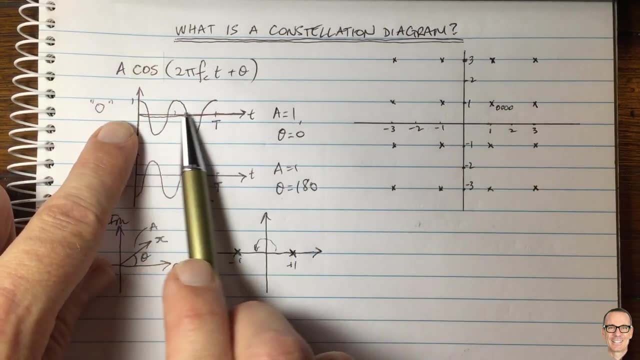 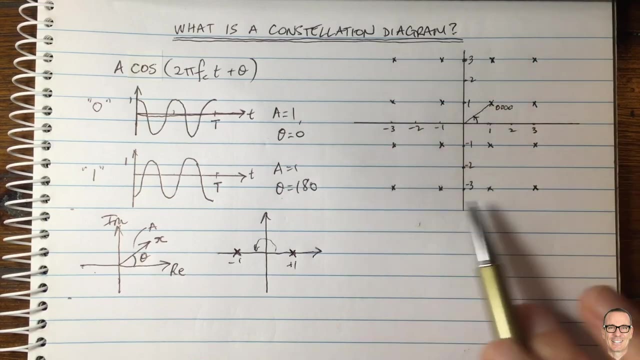 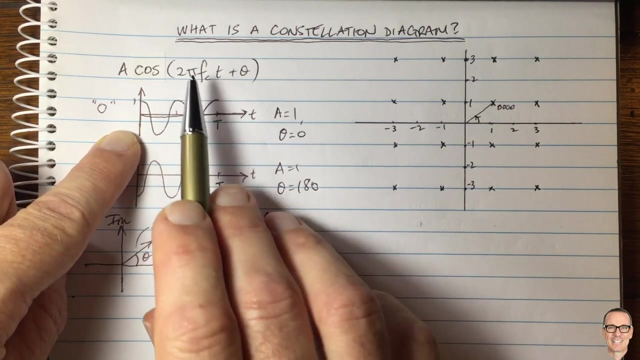 four bits. so example: that could be mapped to 000, mapped to that value of x, And I always encourage people to remember that that value of x means that there's a waveform that has this amplitude here and this phase here. So when you look at constellation diagrams, always be thinking about the waveform that's being transmitted. it's being transmitted for a period of time which you've decided and is fixed, at a carrier frequency which you've been allocated and is fixed, And the choice that you've got is: 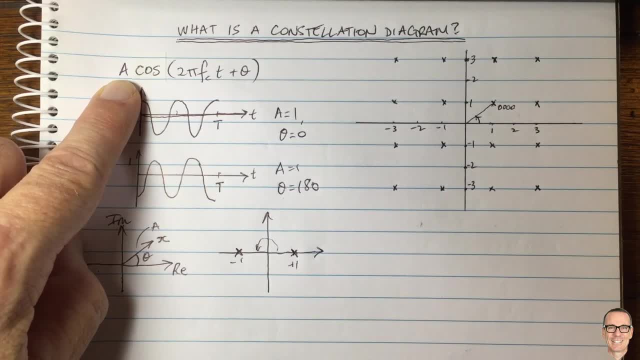 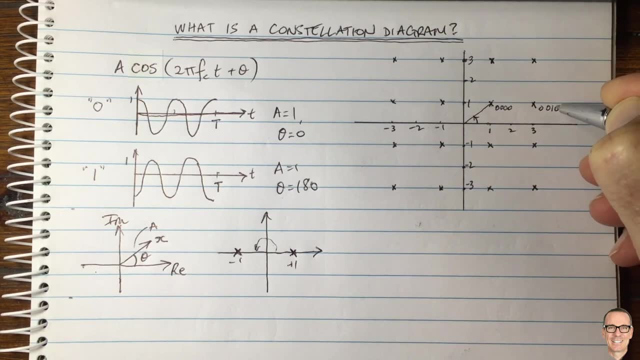 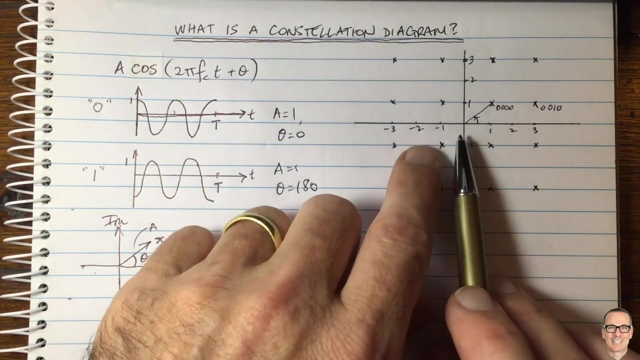 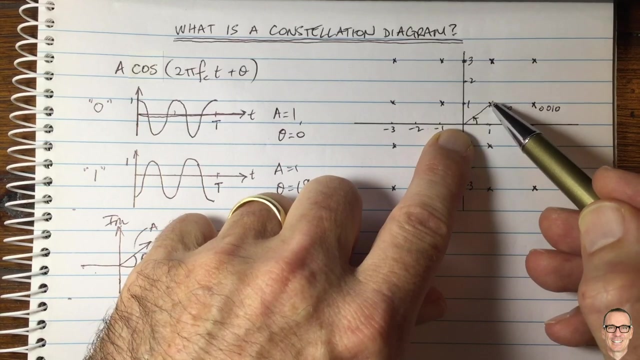 these other two variables, the amplitude and the phase. And so here's, as I say, this one could represent the bit sequence 0010.. And there's some flexibility in the way that you map these sequences to these constellation points. Okay, and here what you notice is: here, these points, here I've put them in a square grid at plus one plus one, So the amplitude here is not one anymore. This is bigger than one, of course, in this case. on this diagram, 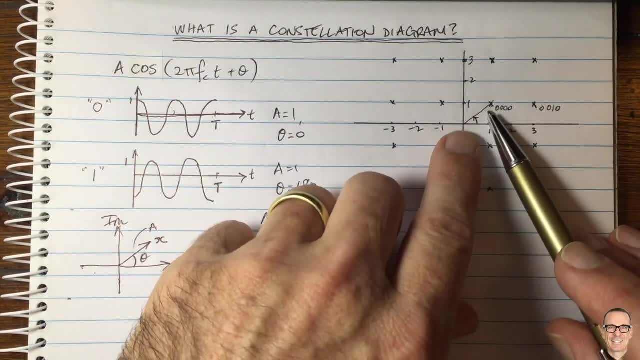 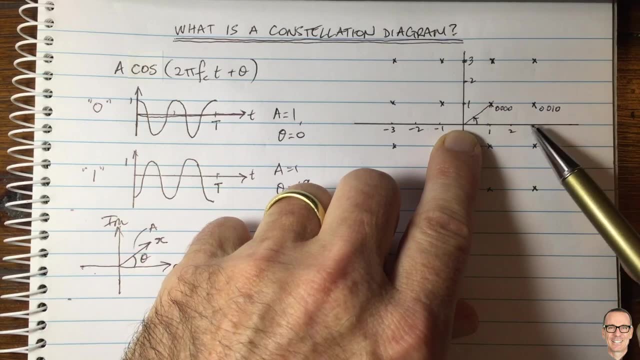 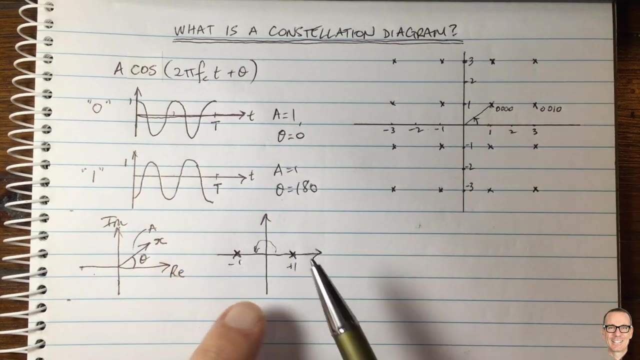 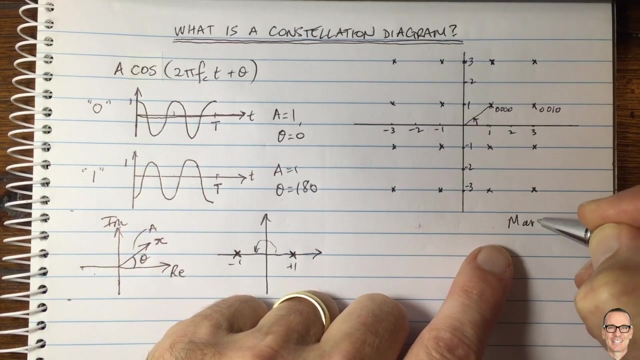 Here they were one apart, So a equaled one over here. a is bigger than one. it's certainly bigger than one for this, because this is out at three, and this is three in the real and three in the imaginary, So that's bigger again. So what do we have to do if we are going to compare these diagrams and decide whether we would like to send binary data or emery data? So this is called emery, emery qam, because it's quadrature. So there's a real and an imaginary. so that's quadrature, And 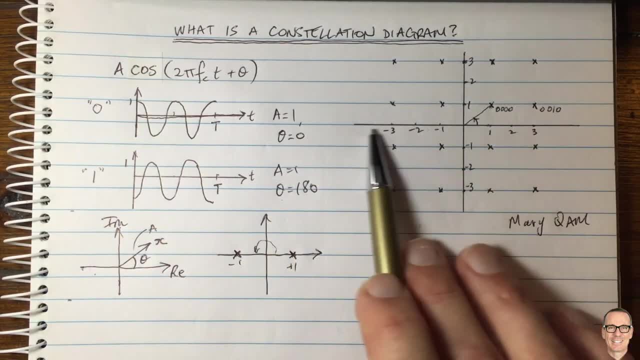 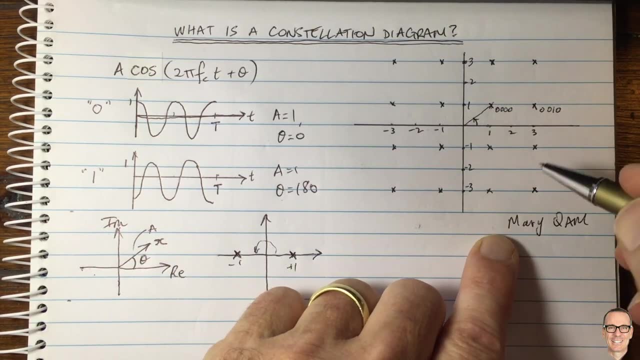 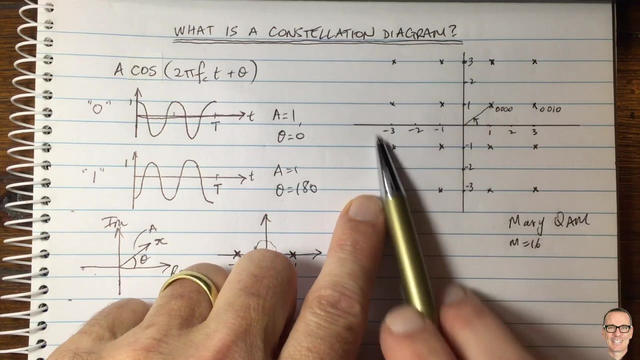 amplitude modulation, because you're modulating the amplitude of the real part and the amplitude of the imaginary part, so that's quadrature amplitude modulation, Emory, in this case 16. so M equals 16 in this particular diagram here. okay, so if you're going to send with this diagram, one important thing: 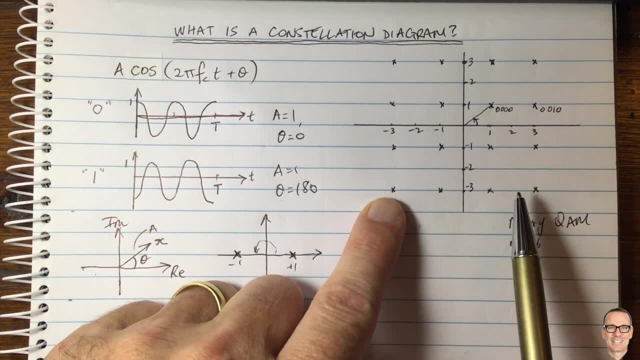 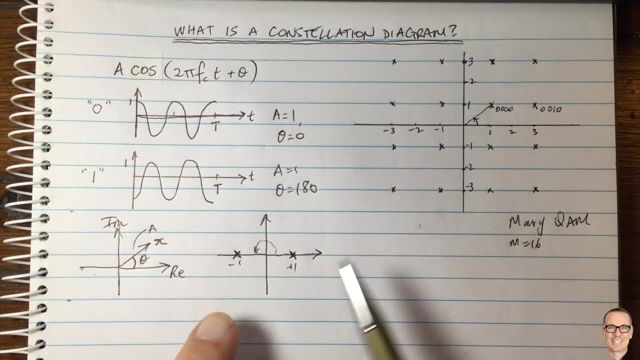 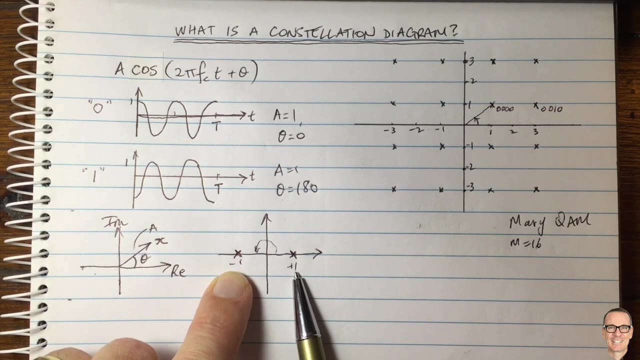 just the last thing to note is you need to make sure that you're comparing for the same transmit power and, of course, the important thing is going to be decoding. how do you decode them and what's the chance of making an error? so in this case, these symbols are two units apart. these are also two units apart, but 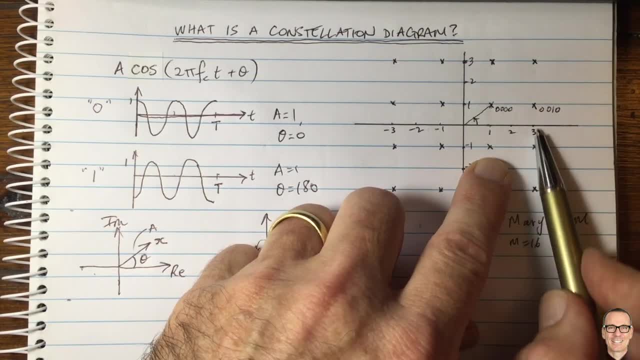 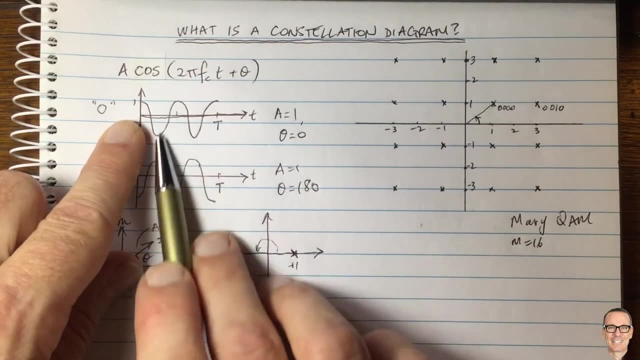 if you were to, all of them are two units apart in the real and two units apart in the imaginary. okay, so that's an important thing. if you're going to receive a waveform like this, it's going to be received with noise and potentially amplified or scaled down because of the channel. 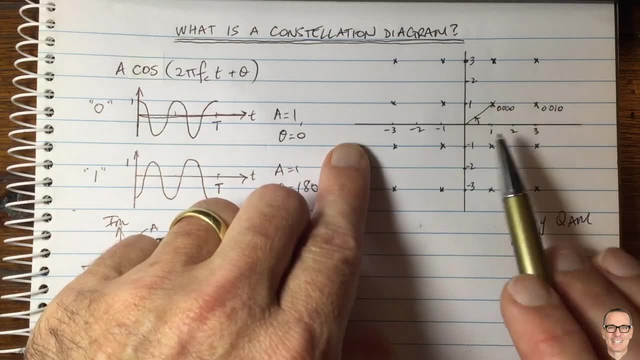 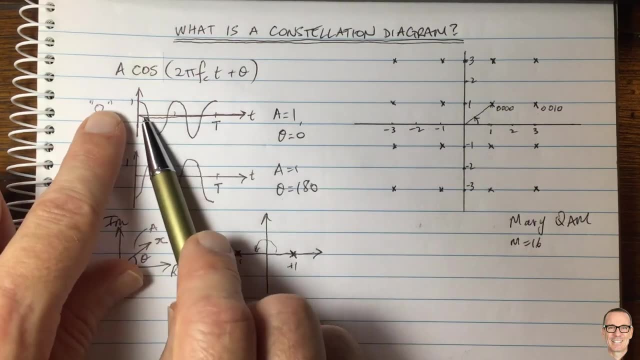 of the wave form and it's going to be received with noise and potentially amplified or scaled down because of the channel losses in the channel. then this constellation diagram is going to be received, squashed in, possibly rotated, and your challenge is to use a matched filter. and there's another video on the. 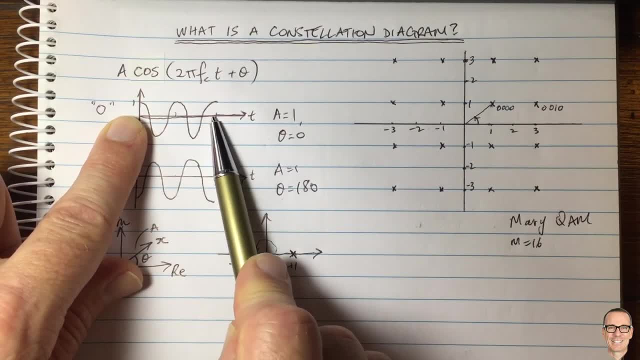 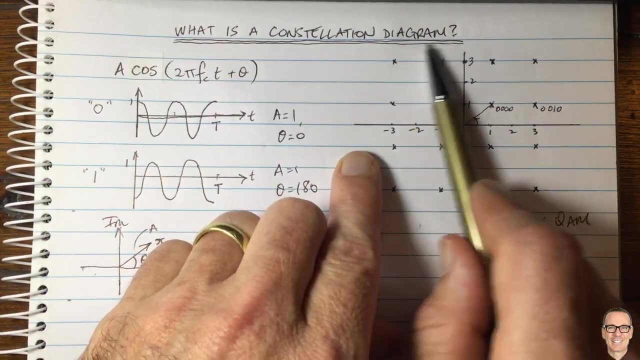 channel about match filters for more information about that, but to use a match filter to map from the received waveform back to the constellation diagram and then to decide which of these actual transmitted constellation points is the one that was received. so it's really important that we get the 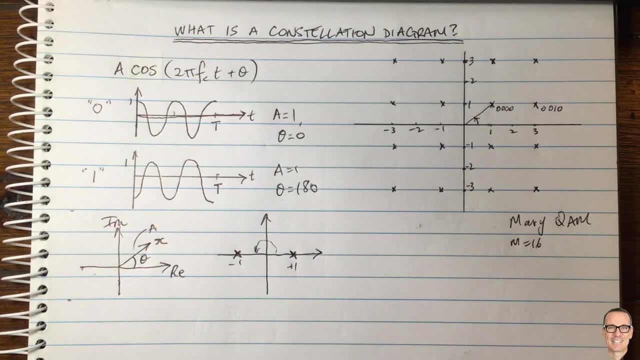 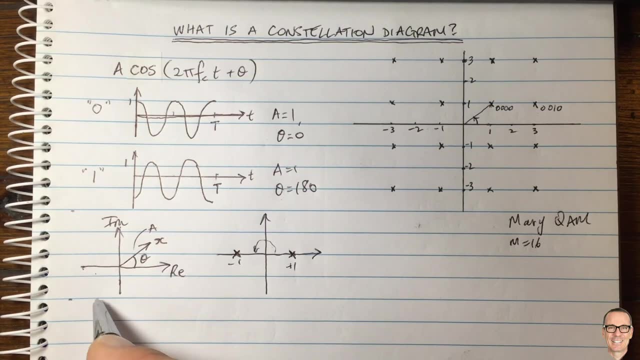 power, correct. so let's just write down the power of this. so the average power is going to be the. so the average power equals the what you're going to. let's write down the power of this waveform here. so it's a squared times cos of 2 pi, fct plus theta. 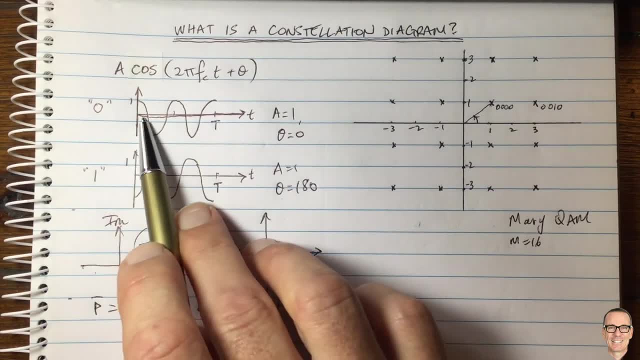 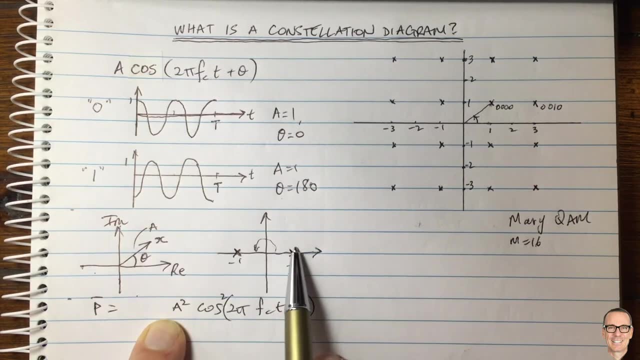 all squared. so the this is the voltage, and you've got to take the square of that to get the power. so now we're going to do this, this for each of the different constellation points you could possibly be sending, or it means each of the different waveforms. So I'm going to do a i and theta, i, and we're going to sum that. 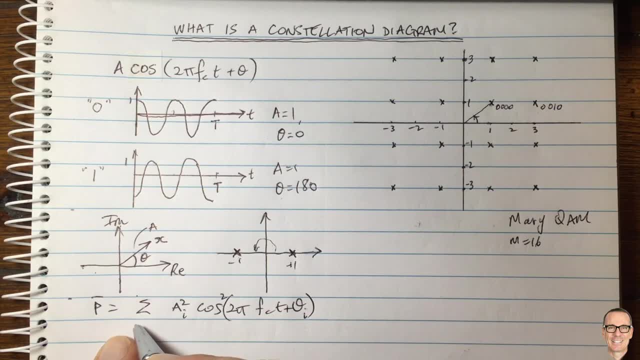 up over all the constellation points. So this is from: i equals one to m, And of course we've got to integrate the energy over all of the time, So from zero time to capital T time. So this is the power integrated over the time and then summed up over all of the different values of m and then 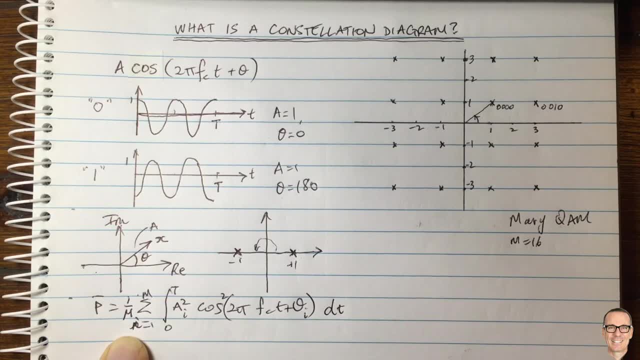 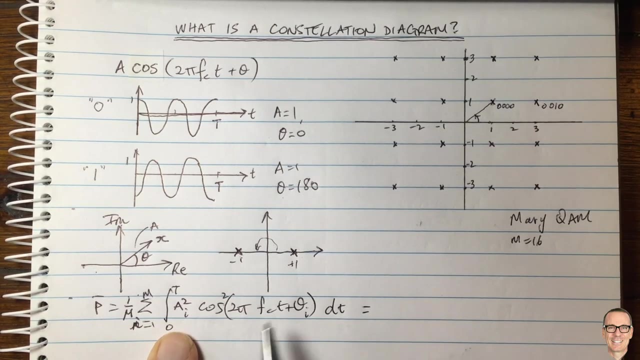 average. we're going to divide by capital M to find the average power, And of course this is going to equal 1, because this part of it, here, this a squared i- comes out of the integral because it doesn't depend on T, And then the integral that's left is independent of or not independent. 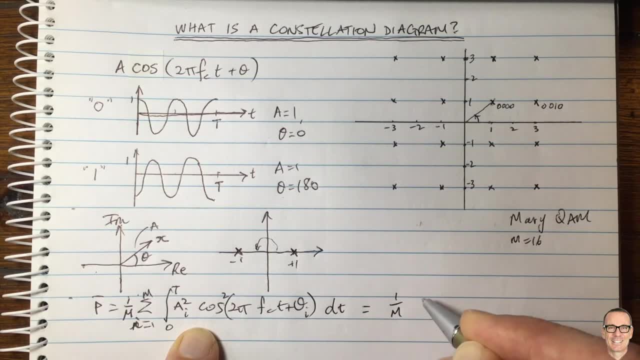 but it's the same for all values of i. So let me just see why that is. So we've got 1 on m. the sum of i's i equals one to m of a. i squared times the integral from zero to capital, t of cos squared. 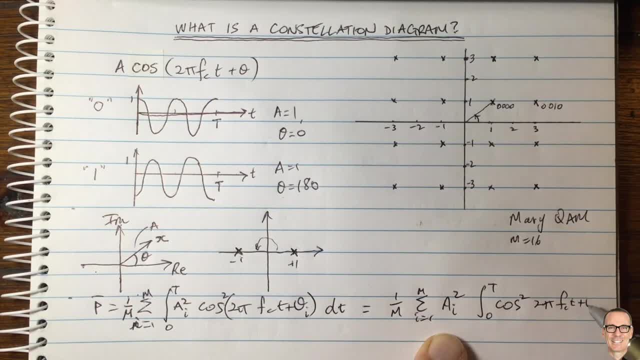 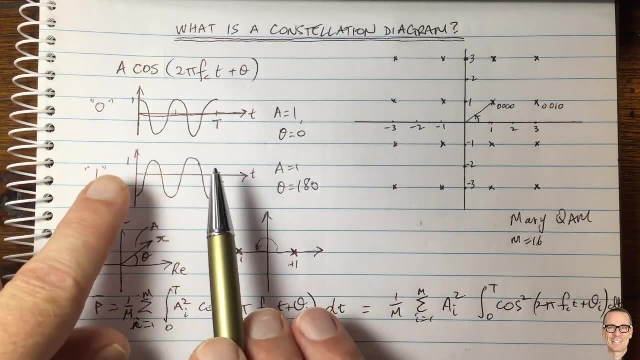 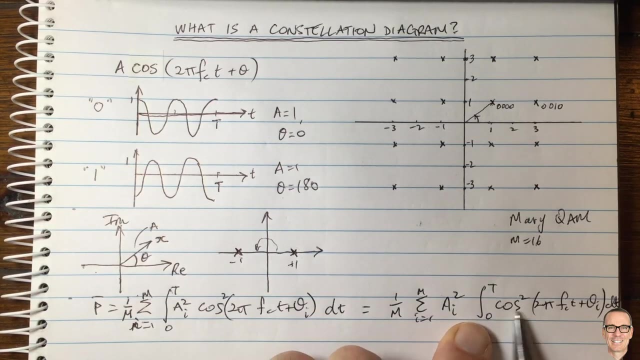 two pi, f, c, t, plus theta, i, dt, and we can see now that all you're doing is changing the phase, which means this waveform is the same as this one, just with a phase rotation, which means when you integrate over an entire period, that value is the same for all of the different phase rotations. 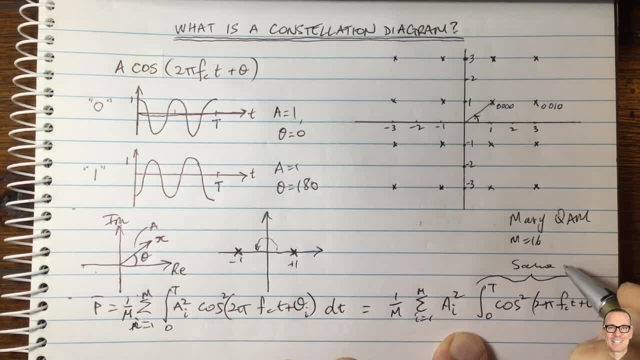 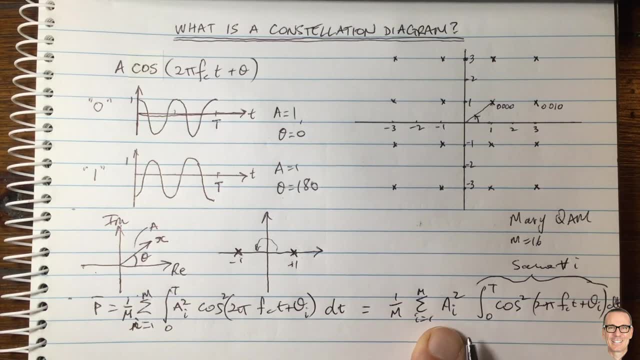 so this is the same for all i, for all i. okay, and this value here, the, the, the um- it's also important to mind. this is also the same for all values of m, okay. so if we're going to look at now our signal, let's look at our what's actually received and what's transmitted, then we're going. 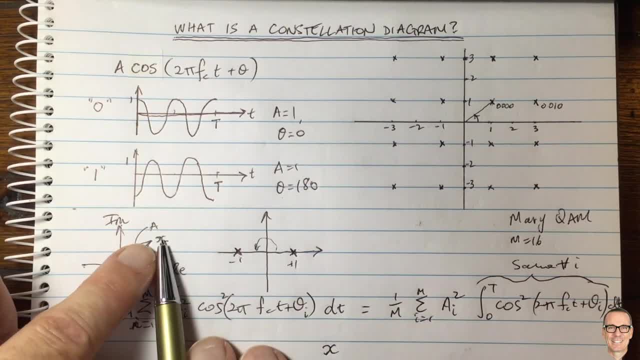 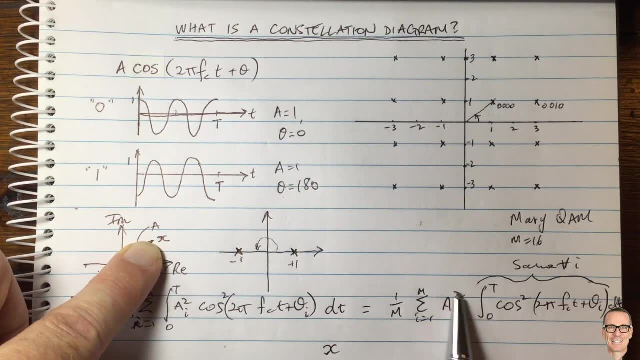 to be transmitting our value x in the baseband. we can, we can use this uh now, because this is the same for all i. we can now focus on what's actually received and what's transmitted, so what we call the baseband, which is this component, which involves this component here. 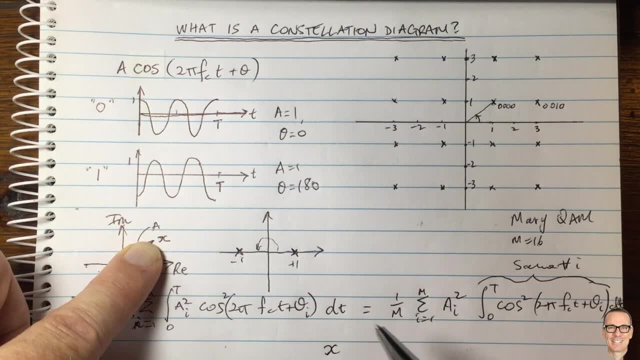 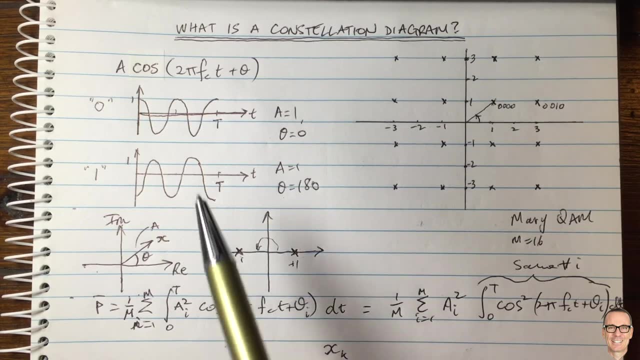 and we're just using x to represent this, which we know is a, is an accurate representation. so it's a sufficient representation in the baseband. so if, at time, little k, you're going to send one of these constellation points, it means you're sending one of these waveforms. then we're going. 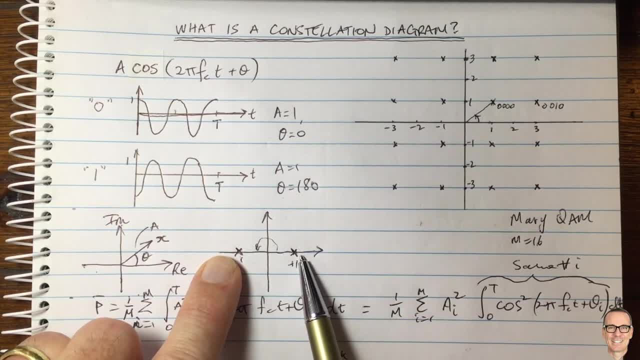 to scale that because it's coming from this constellation point here, which is plus and minus one, and this one goes all the way up to three. we need to make sure we're sending with the same power. so we're going to send one of these waveforms and we're going to send one of these waveforms. 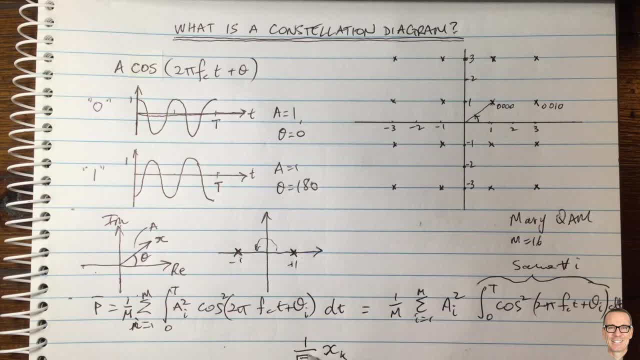 so we need to normalize this over p. so you take this constellation point and you divide by the square root of the average power and this will give you a constellation point which is, on average, the same if you use this constellation, or if you used this constellation, so this gives you a power. 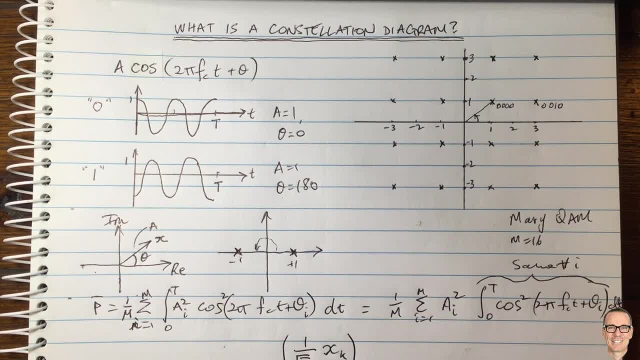 of one, and then, of course, we might want to transmit that with, with, with a power that our transmitter has. so this means we can compare across different modulation formats equally, you're going to, you're going to have a transmit power of one, and then, of course, we might want to transmit that. 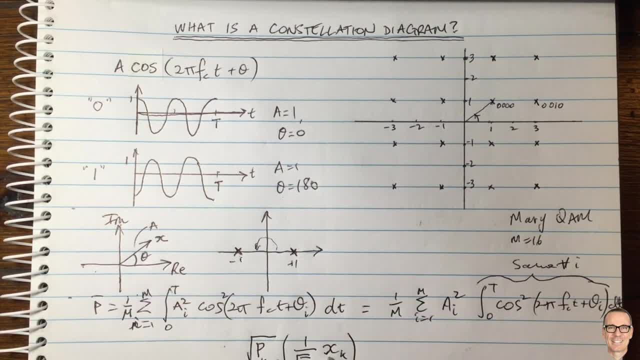 with just the power which you need to multiply by this, this signal, by the square root of that transmit power, so that when you take the square you get the transmit power, because this has unit power, and then of course you might have a channel gain, and then you're going to. that's what you're going. 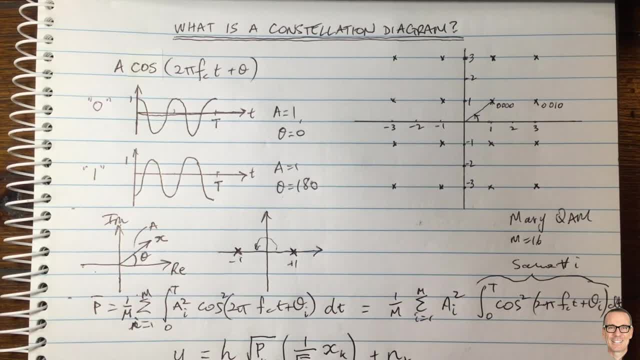 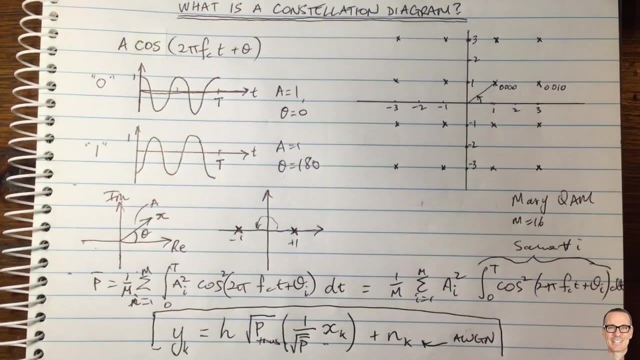 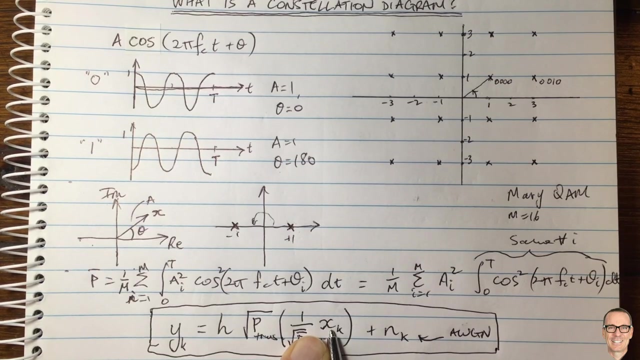 to be receiving. of course there's going to be also white gaussian noise in most channels, additive white gaussian noise in the receiver, which comes from the receiver electronics in your in your receiver equipment. Okay, so this equation here is the equation for the transmitted signal, where xk is a represented in the baseband. it is one of these constellation points and if you scale, 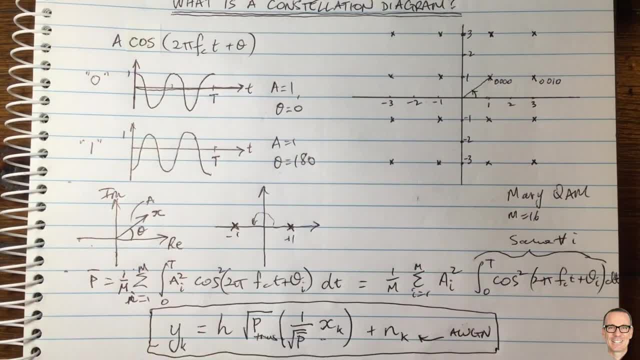 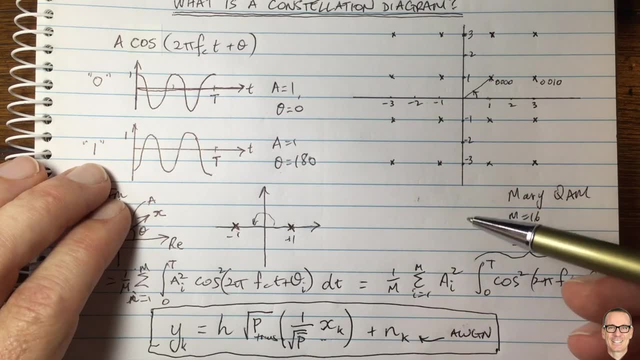 it with this power. that means you can compare different constellation points equally, So hopefully this has given you more insights into the constellation diagram and the role it plays in digital communications. If you like the video, give it a thumbs up. it helps others to find the 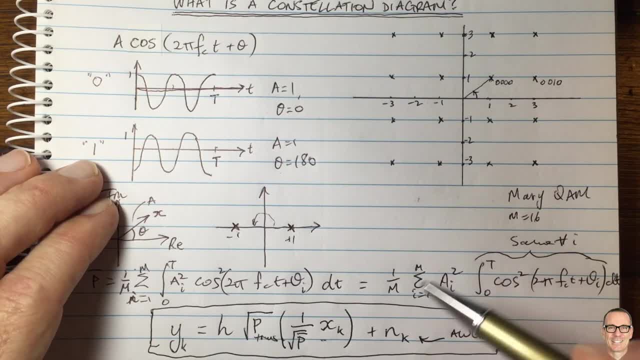 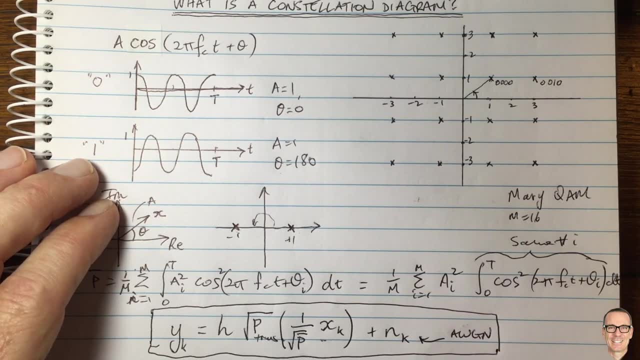 video. Subscribe to the channel for more videos and check out the web page in the link below, where there's a full categorized link of all the videos on the channel.